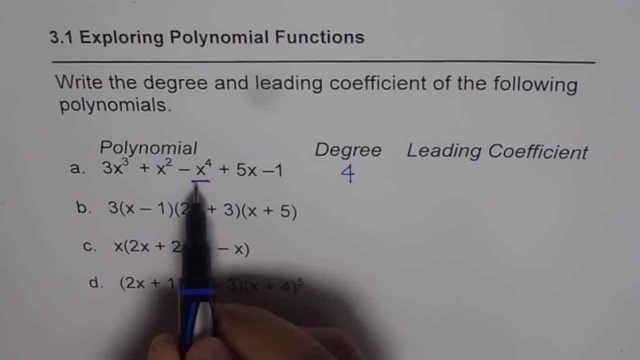 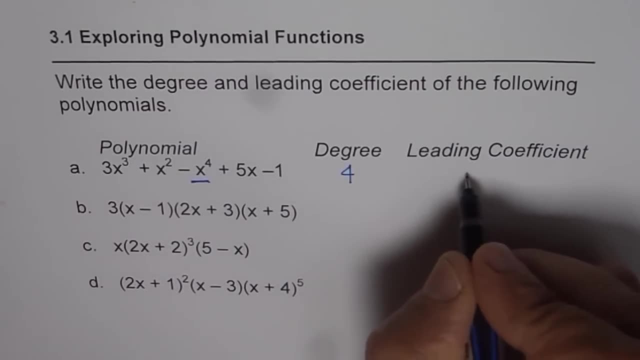 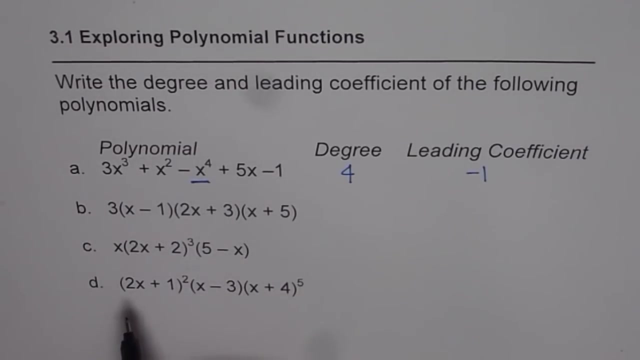 Leading coefficient is coefficient of the term with highest degree right. So this term has a leading coefficient of minus 1.. Okay, so that's the first one. The second one is: we have given the polynomial in factored form. Now you don't really have to multiply, expand. 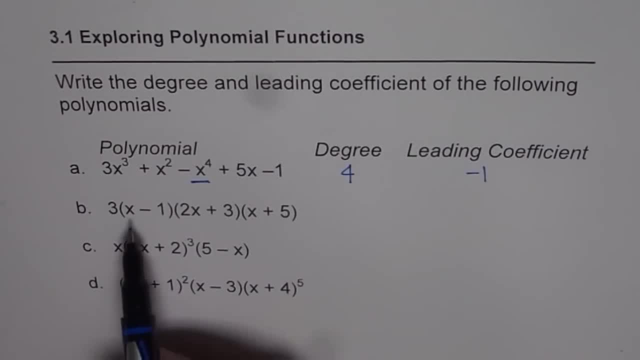 get to this stage and then find the answer. You should remember: if you multiply x with 2x, you are going to get 2x square 2x square times x will give you 2x cube. Don't forget about 3 here. So that should give you 3x cube. 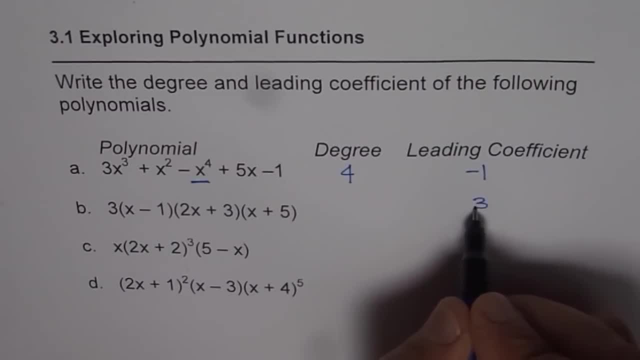 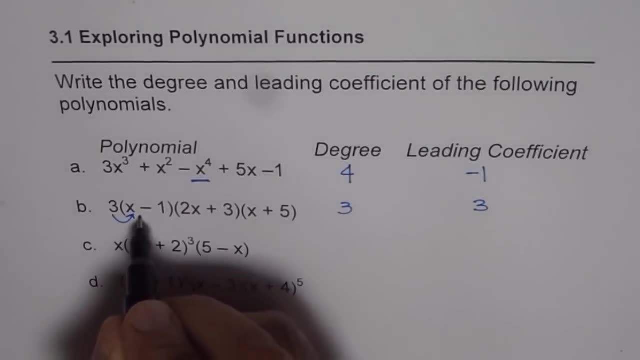 right. So 3 becomes the leading coefficient and 3 becomes the degree, the x cube term, right? So you've got to multiply 3 with this x, These terms, These terms, when multiplied, will give you the leading term from where you can find degree and the leading coefficient. 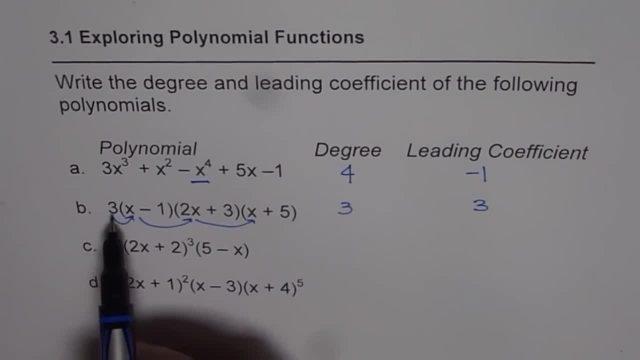 right. I think I did something wrong. Let us do it again. 3 times x is 3.. 3 times 2 is 6.. So it should have been 6, right? So leading coefficient is 6 for us. Now let's get to. 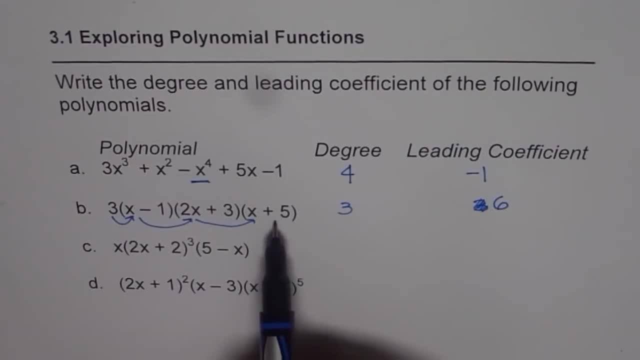 C. Now we will apply the strategy learnt here and then write down degree and leading coefficient of part C. Now, purposely given this, do you see that minus with x It makes a huge difference And the cube here will make it 2x cube right. So, in a way, what are we multiplying to get? 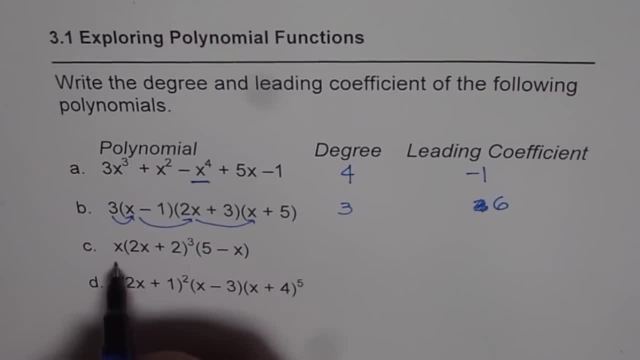 the leading coefficient. Let me show that. So we have x times 2x cube, right? So we should write 2x cube here and then minus x. Do you see that Now degree will be 1, and then 1, plus 3,, 4, plus 1,, 5.. So degree for us is 5. And the leading coefficient is 1 times. 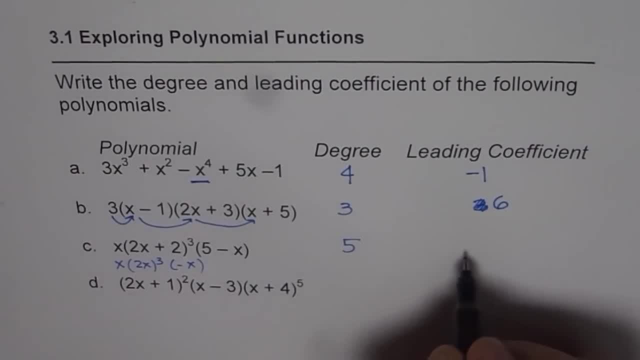 2 cube, which is 8 times minus. So it is minus 8.. Now the last one. here is given in factored form Degree. you can count When you multiply them: 5,, 6, and 1, and 2, 8.. So the degree is 8.. It's an even degree function And leading.